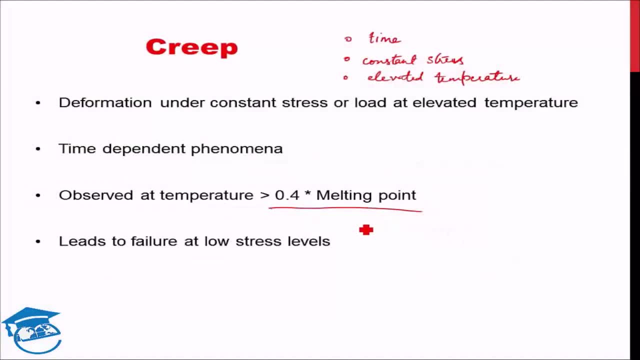 melting point. So there is no hard and fast degree Celsius boundary, rather there is a dependent on the melting point. Now what happens is that under normal circumstances, if you do a tensile test below this temperature, you will have a temperature of 0.4 times its melting point. So the temperature at which 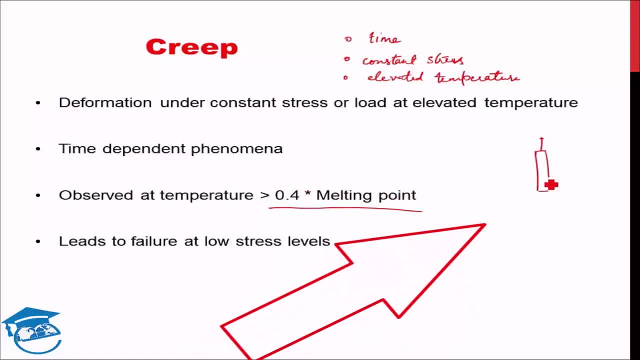 creep occurs is normally in the range of 0.4 times its melting point. So there is no hard and fast degree Celsius boundary. So what happens is that under normal circumstances, if you do a tensile test below this temperature- suppose you provide stress- then for a given 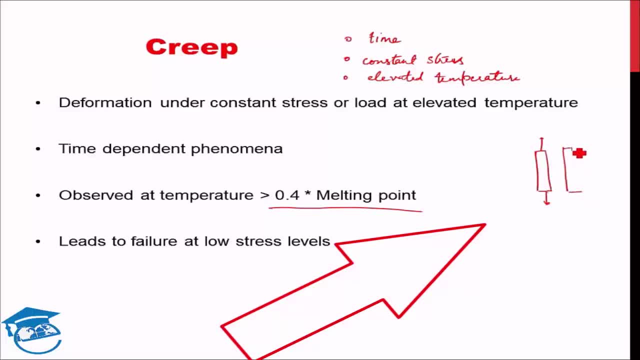 stress, it will elongate to a particular length and if you do not change the stress any further, then it will remain at that length, right? In order to further elongate it, you need to increase the load or you need to increase the stress, But that is not the case when. 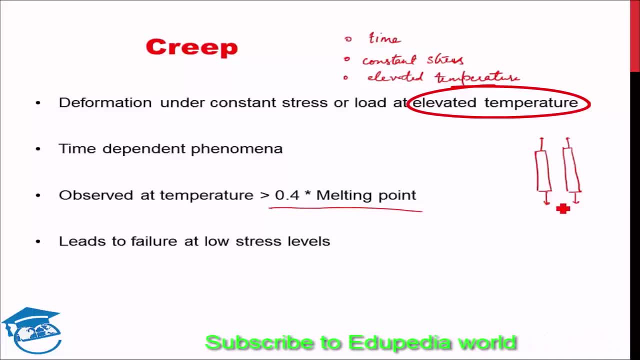 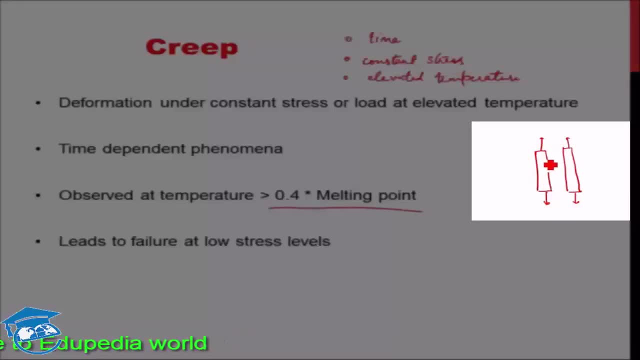 we are talking about elevated temperature. The temperature at which creep occurs is normally in the range of 0.4 times its melting point. The temperature at which creep occurs is normally in the range of 0.4 times its melting point temperature. what happens is you have a particular stress. you keep the body at a 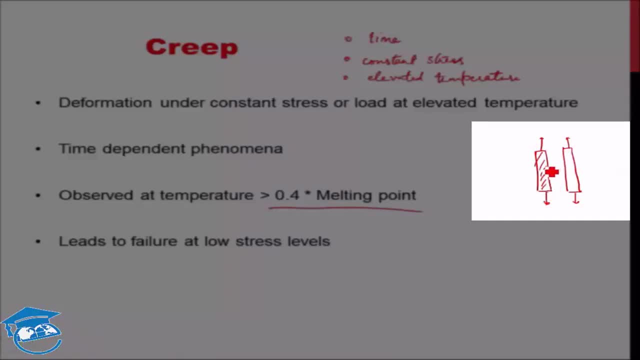 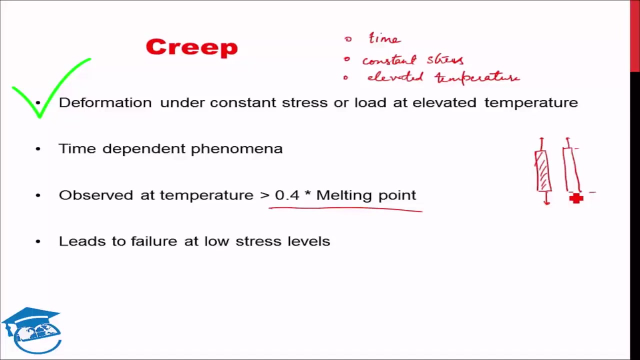 higher temperature. at that stress the body keeps on elongating with time. it is not reaching a particular elongation and stopping there. so creep is basically deformation under constant stress or load at elevated temperature which continues with time. therefore it is a time-dependent phenomena. at one time it 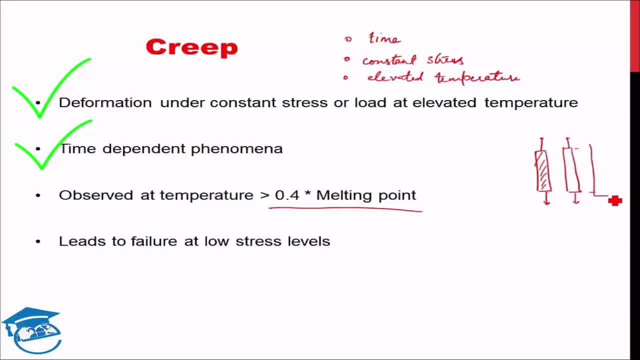 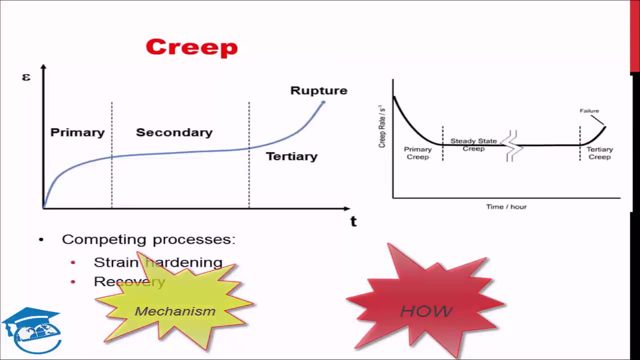 is at this length under the same stress. after some time it will increase further, so it is a time-dependent phenomena. now let us see how does creep happen, or what is the mechanism behind creep happening. so creep basically occurs in three different stages. okay, one thing this should start from: 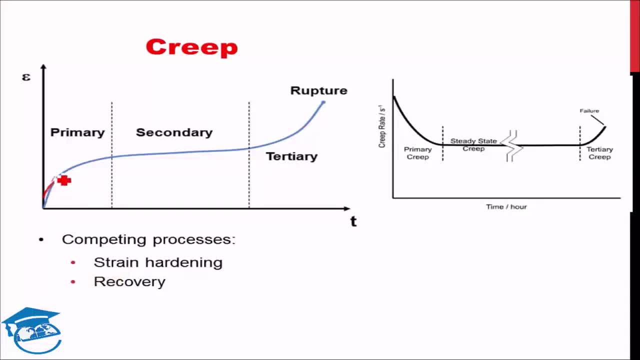 somewhere like this. so creep basically occurs in three different stages. okay, one thing: this should start from somewhere around here, not zero. okay, this is the instantaneous elongation which takes place as soon as you load the material right. so here, what we see is that there are three stages of creep. there is a primary region, a secondary region and a 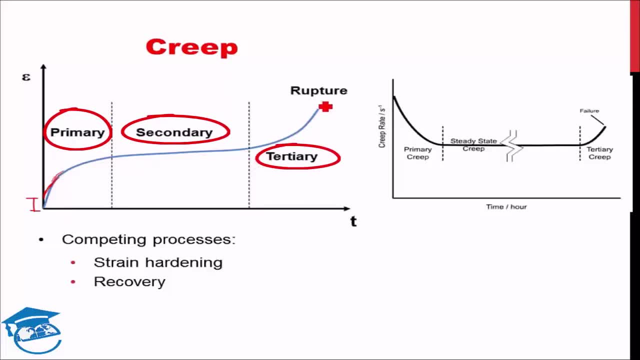 tertiary region. the tertiary region ends up with failure, or alternatively known as rupture. the secondary region is the longest region. this is not to scale. this region is actually much longer compared to region 1 and region 3. okay, so the secondary region is the major region and this region has a constant creep rate. 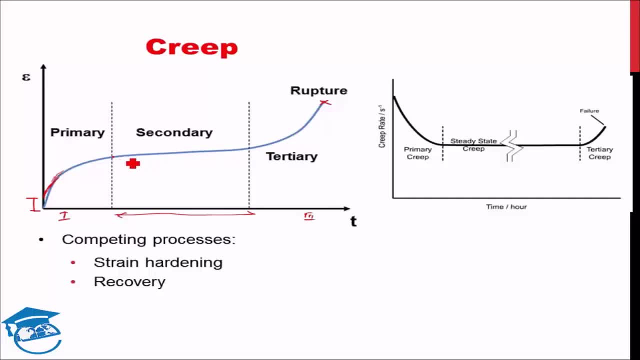 that the, that is, the change in strain, is constant with time. data of change of strain is constant. Primary region: the creep rate is maximum at the beginning and it keeps on decreasing, decreasing, decreasing, reaching a minima. here That creep rate continues in the secondary region. It reaches a threshold and then 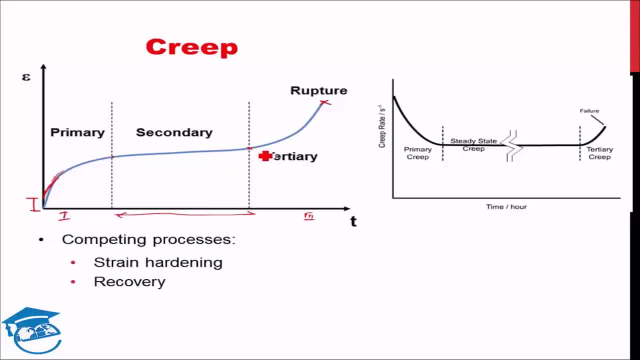 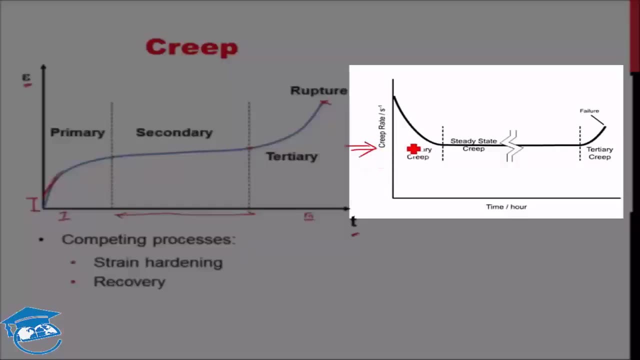 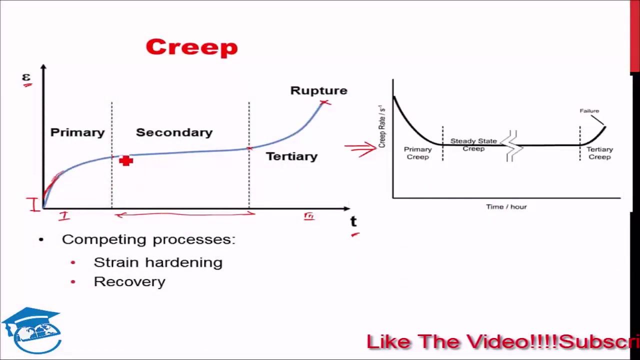 the tertiary creep starts, where the creep rate again starts to increase, increase, increase and suddenly there is a rupture. So this graph is basically strain versus time and we have converted this to strain rate or creep rate versus time over here. Similar: in the primary region, the creep rate was decreasing. 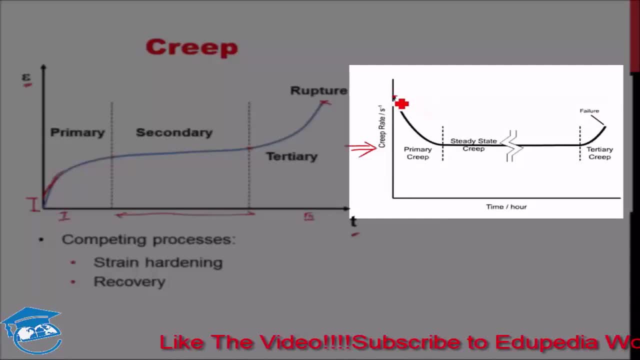 continuously Here. initially the creep rate is very high. it decreases, reaches a threshold, a minima, a steady state creep rate, and then the tertiary creep starts, Creep rate is obtained and that creep rate goes throughout the secondary region. Then the creep rate starts to increase. Okay, so there are two competing. 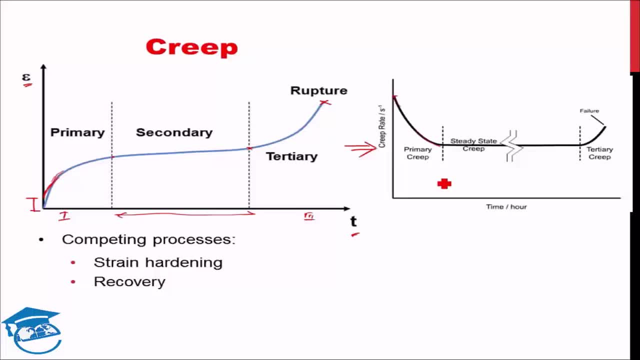 processes going on during creep, that is, deciding the creep rate. What are the two competing processes? The first process is strain hardening and the second process is known as recovery. Let us understand both the processes separately. Strain hardening: what does this do? is that it 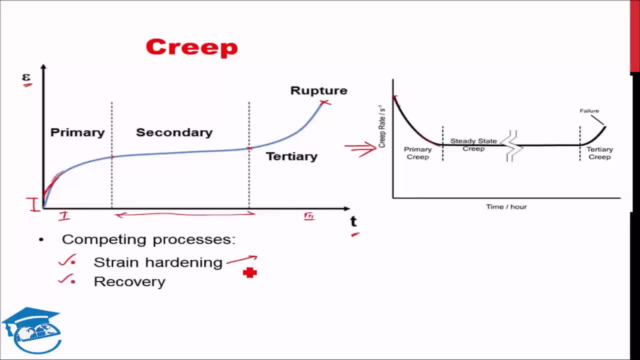 makes it difficult for the material to creep further, That is, to elongate further. It basically hardens the material. Okay, it hardens the material due to the strain which is developed. The strain tries to restrict further elongation, further change in dimension. So this is known as strain hardening- It hardens. 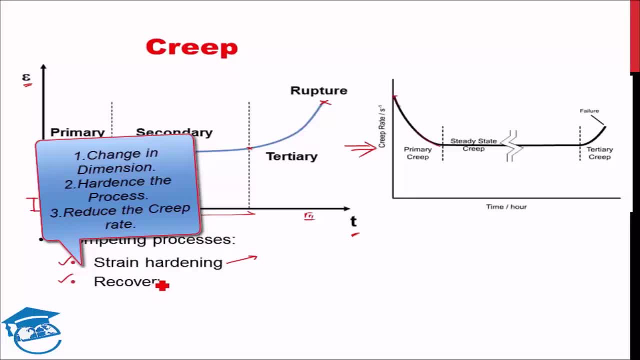 the process for from occurring further. Therefore, this will try to reduce the creep rate, isn't it? Whereas recovery is a softening process, It softens and thereby it kind of tries to increase the creep rate. It makes the movement of dislocations, which we'll see later, easier, Thereby making the creep process. 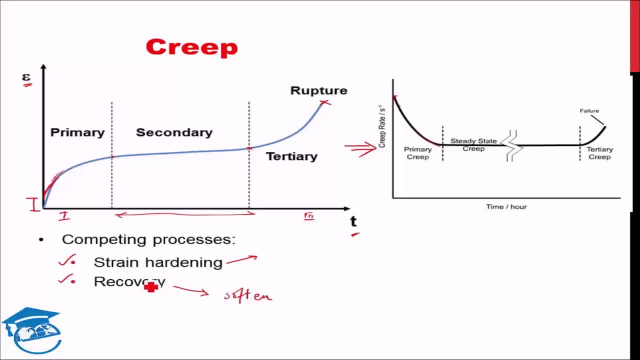 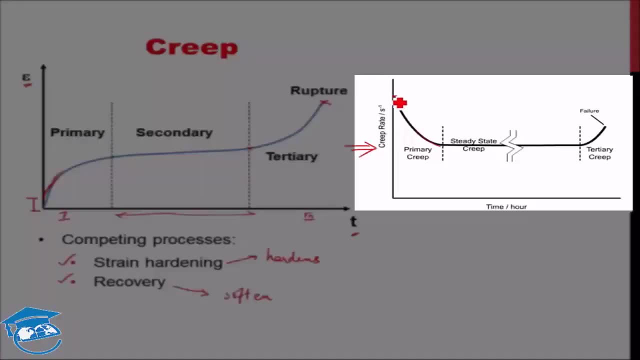 easier. so these two are opposing processes. this hardens, this softens. now, what is happening over here? over here, initially there is no strain within the body, right, but as soon as then material begins, begins to strain, the material begins to strain, harden. as a result, the strain hardening takes over. it is the effect of 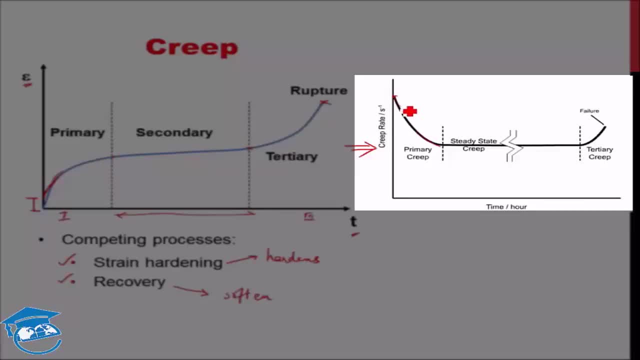 strain hardening is more than the effect of recovery, and the materials creep rate keeps on decreasing once it reaches this point, once it reaches the end of the primary zone, the rate of strain hardening and rate of recovery becomes equal. when that happens, what happens is the rate of hardening and rate of 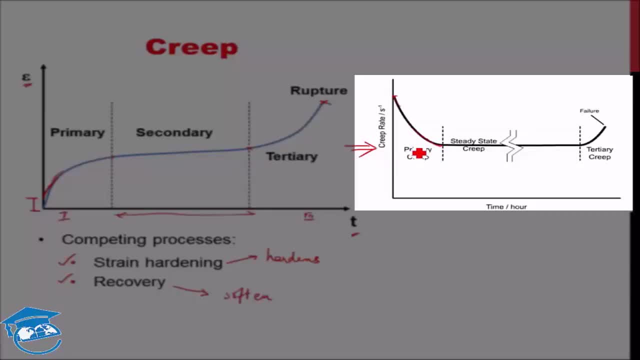 softening becomes equal and we reach a steady state of creep rate. therefore, this whole second state of hardening is the rate of recovery and the rate of secondary region is steady state creep because strain hardening rate and recovery rate are the same over here. here what happens? you end up with some 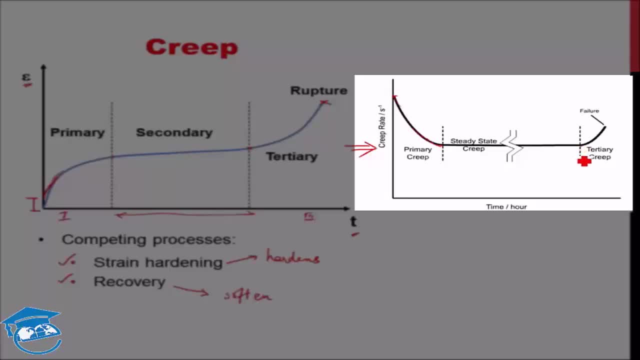 voids or some cracks or some necking, whereby the strain creep rate again starts to increase. so basically, internal discontinuities, internal fractures, internal cracks begins to grow over here and, as a result, the tertiary creep starts to pick up, the rate creep rate starts to pick up and finally it. 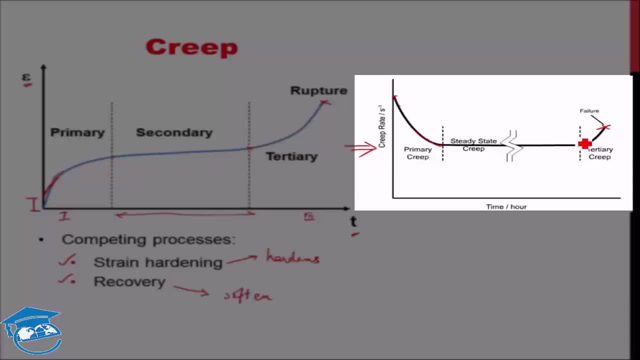 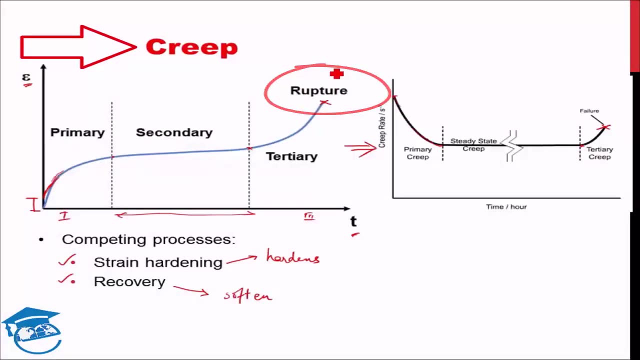 leads to the failure of the material, alternatively known as a rupture of the material. so this is the whole process of creep. this happens only at elevated temperature. if the material notices this right after the material is out of the was not at a elevated temperature, then for a given stress, what would have? 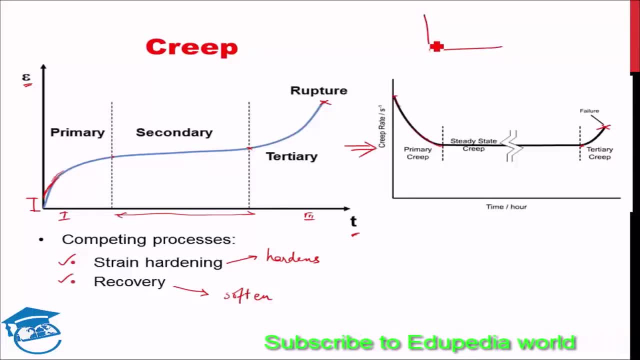 happened is it would have got a particular elongation and stopped over there. so what would have happened is: stress is here, rather, strain is here and time is here. if the stress remains constant, then the strain will also remain constant with time. stress is equal to constant, but this happens at. 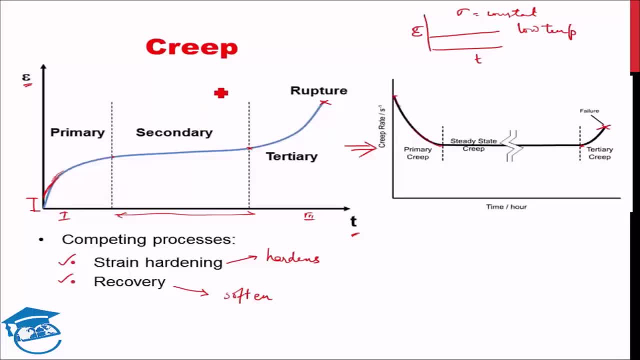 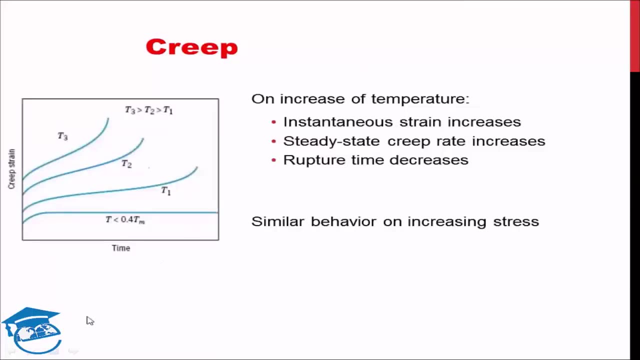 low temperature. this happens at elevated temperature. fine, now let us see what are some of the properties, or what are some of the factors which influences creep. what is the influence of temperature on creep? if we increase the temperature, what will happen is that the instantaneous strain will increase. what we see here is: T1 is the smallest and T3 is the largest, so on. 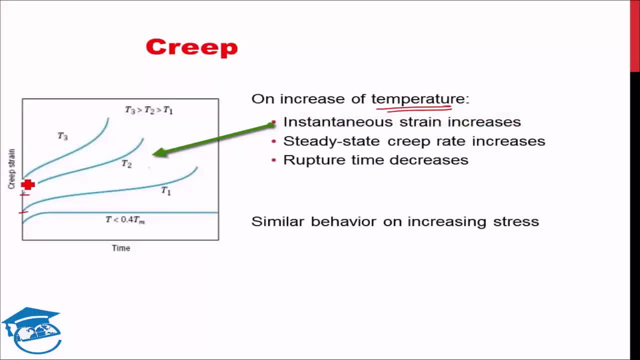 increasing temperature, the initial strain, instantaneous strain, keeps on increasing. this is the first thing which will observe on increasing temperature. second thing which will observe is that the steady state creep rate also increases with increase in temperature. here the steady state creep rate is this slope. so basically, this slope is increasing with increasing temperature. 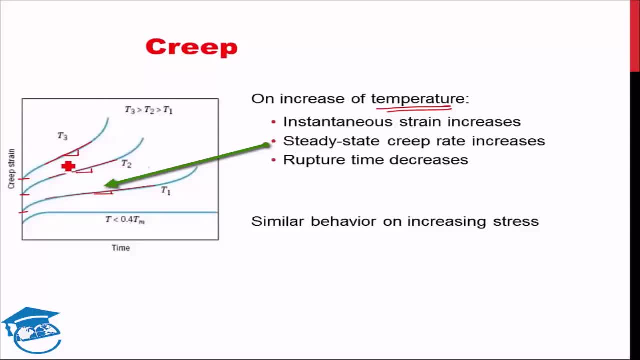 for the steady state creep rate, that is the secondary stage. creep rate is increasing with increasing temperature. Finally, with increase in temperature the rupture time is decreasing. higher temperature, more creep happening per unit time. therefore rupture happens faster. this is time scale. so for t1, which is the lowest temperature, rupture is happening here with